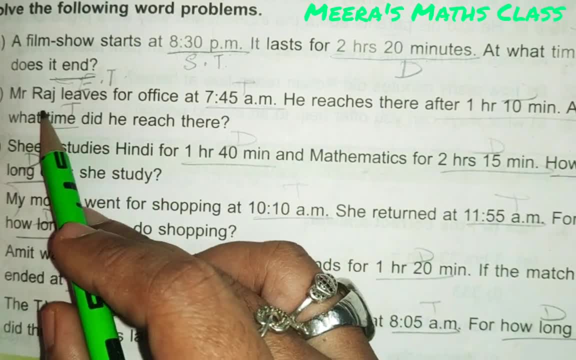 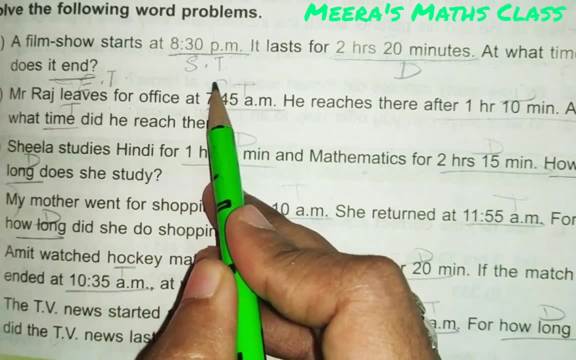 I'll read one more question to make you understand. Mr Raj leaves for office at 7.45 am. That means starting time. Write ST. Underline and write it ST. You can write it on the top or below, That doesn't matter. 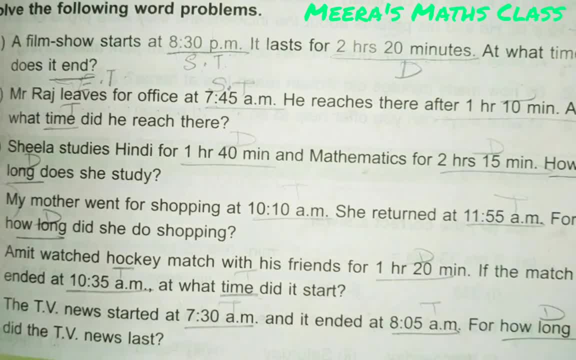 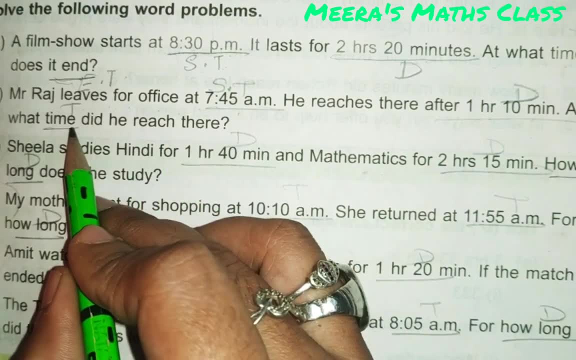 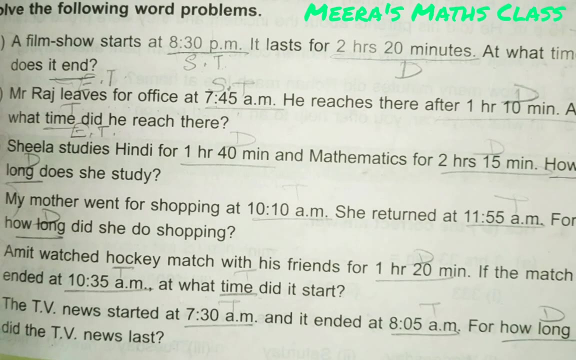 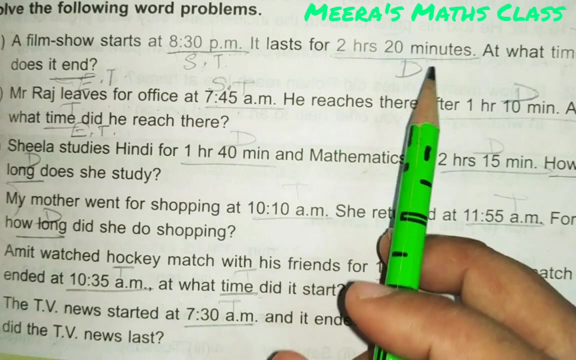 He reaches there after 1 hour 10 minutes. That is duration. At what time did he reach there? That means which time it is asked. This is end time, Okay. So now let's do these two questions first, Where starting time is given and duration is given. 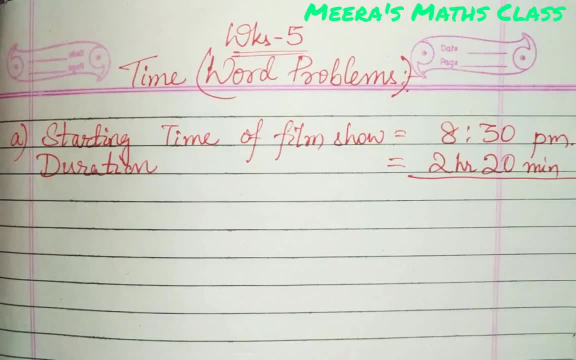 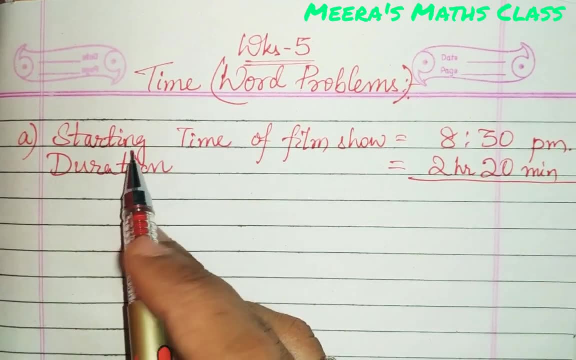 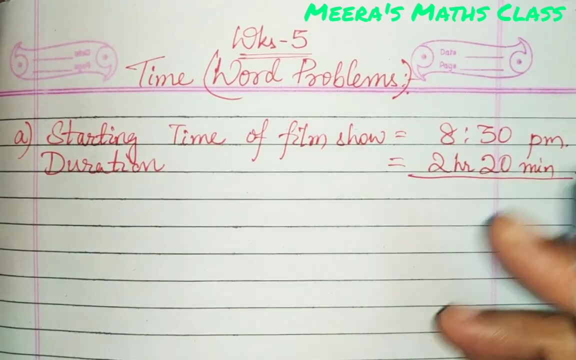 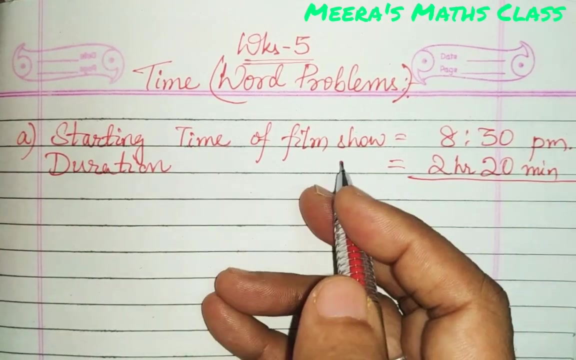 And end time is asked. Okay, So here you see how to write. Starting time of film show is equal to 8.30 pm. Now what is the duration the movie runs for? or the film show runs for? Duration is equal to 2 hours and 20 minutes. 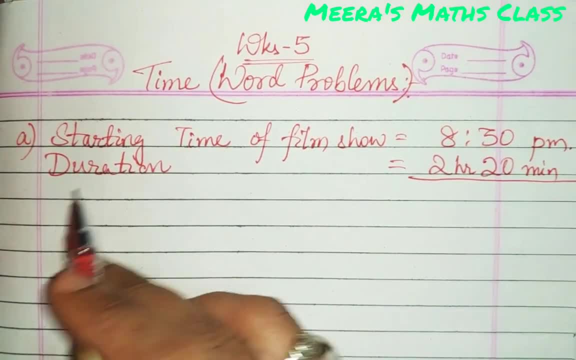 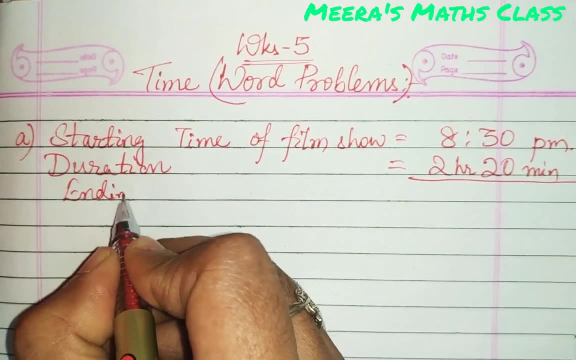 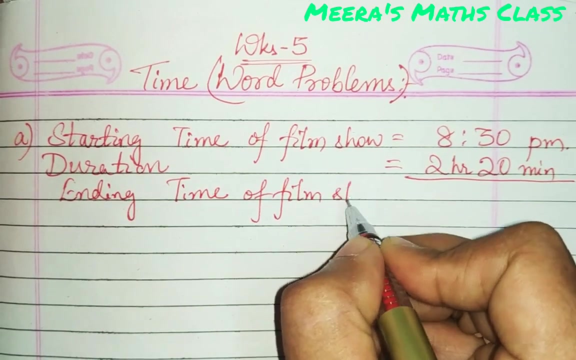 Now, here, starting time is given, Duration is given. What you are going to do: You are going to find out the end time, Or you can write ending time When it is ending time of film show. What you are going to do here. you are going to add it, okay. 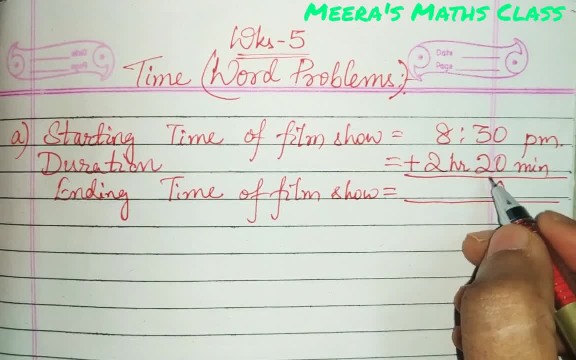 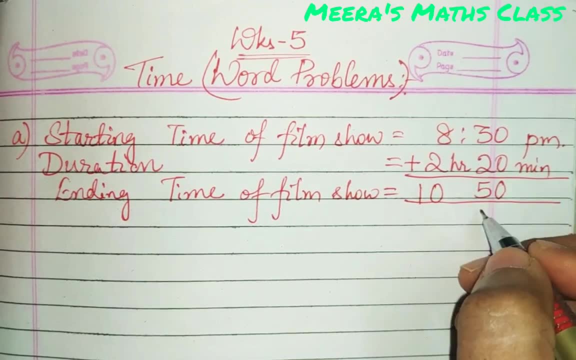 So let's add it: 0 plus 0 is 0,, 3 plus 2 is 5,, 8 plus 2 is 10.. Now what will you do here? Don't write hours and minutes. This is ending time. 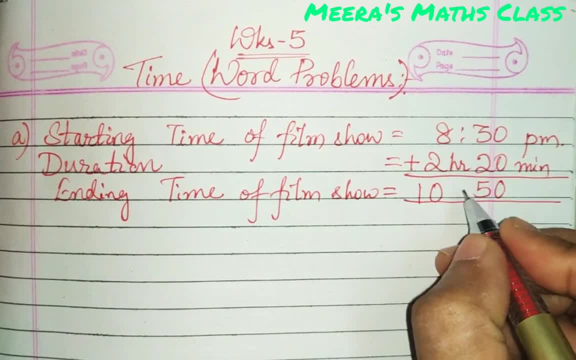 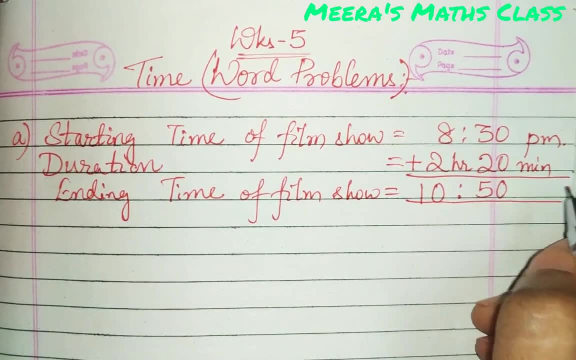 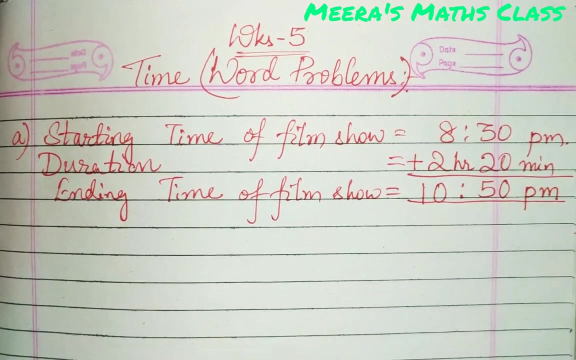 It will be am or pm. Remember that. So 10,, 50, here pm is given. So 8 to 10,. there is no 12 o'clock area. I mean 12 numbers, Number in between. So you will write 10,, 30,, 10,, 50 pm. 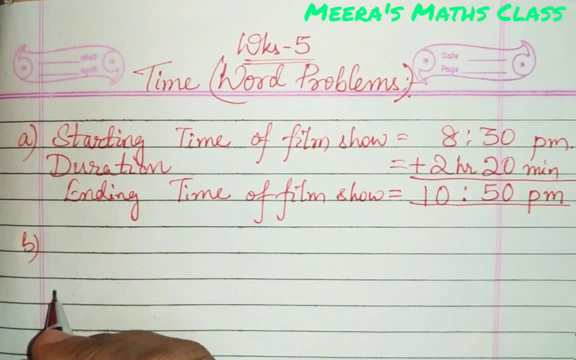 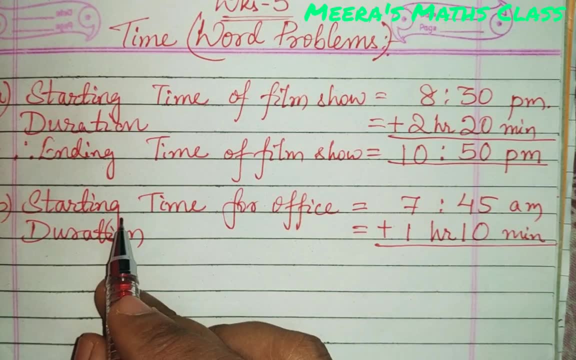 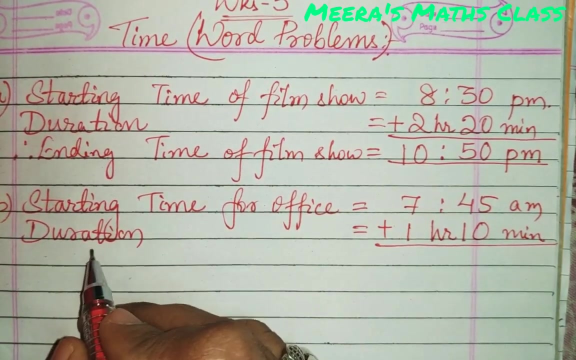 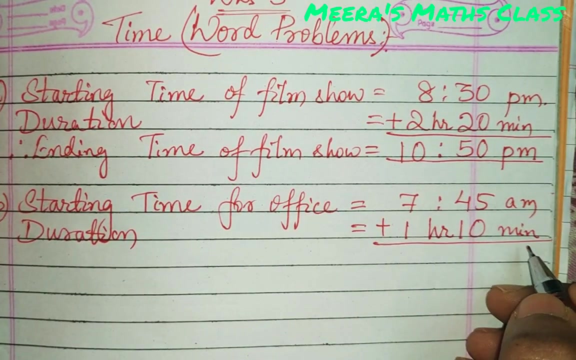 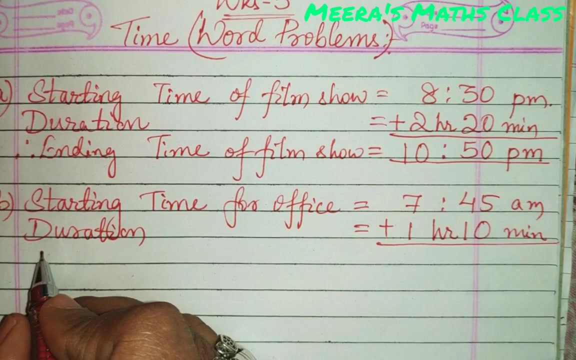 Now similarly for b number. Let's write. So now you see. Starting time for office is 7.45 am. Then comes duration: 1 hour 10.. 10 minutes After completing the distance when he is reaching the office. what will be the time? 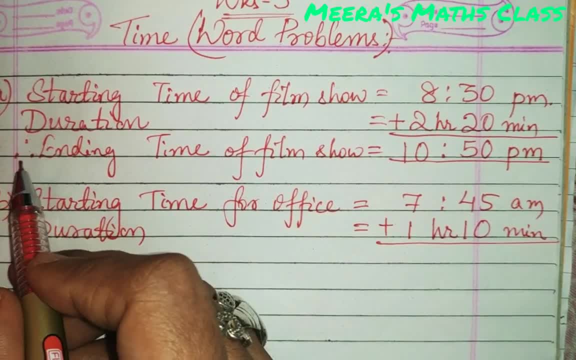 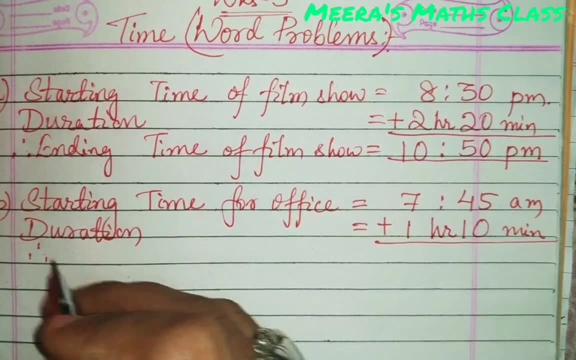 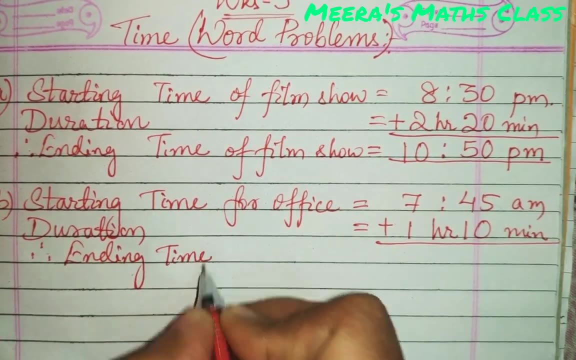 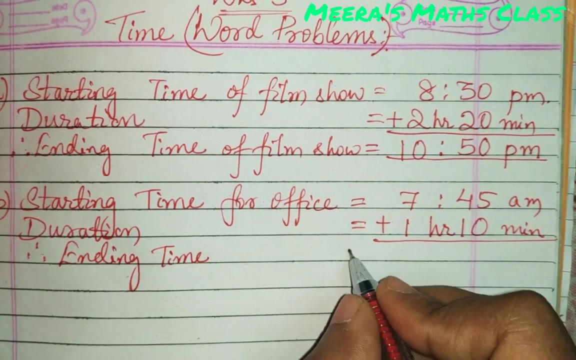 Therefore, yes, I forgot to tell you to put the therefore. here You put: therefore, ending time of film show is 10.50 pm. Now, therefore, ending time 10.50 am is equal to Okay, Is equal to. 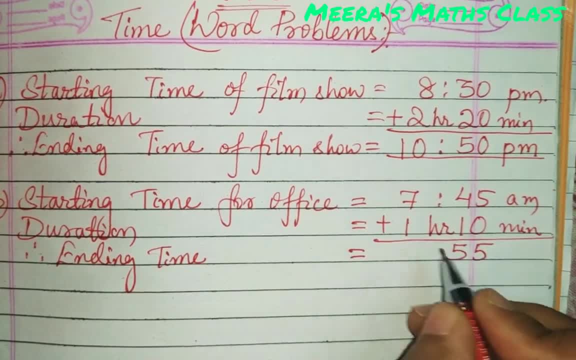 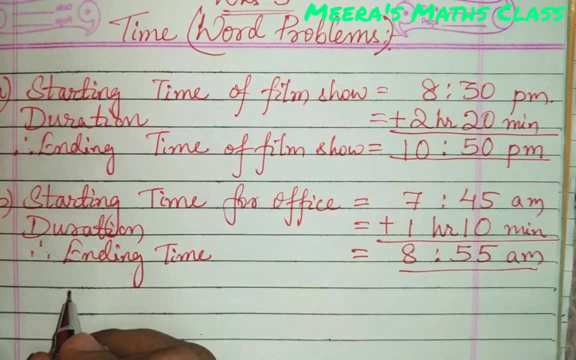 You have to add 5, 4 plus 1, 5, 7 plus 1, 8.. So 8, 50, 5 am. You can write After this. you can write a sentence even: 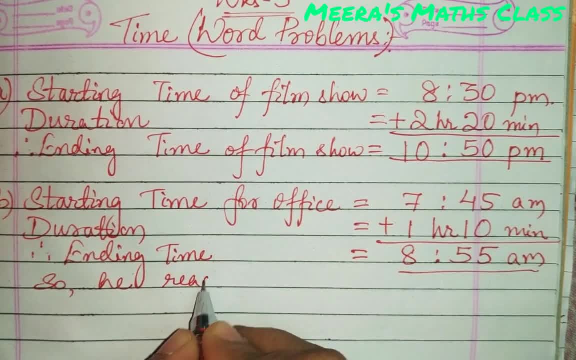 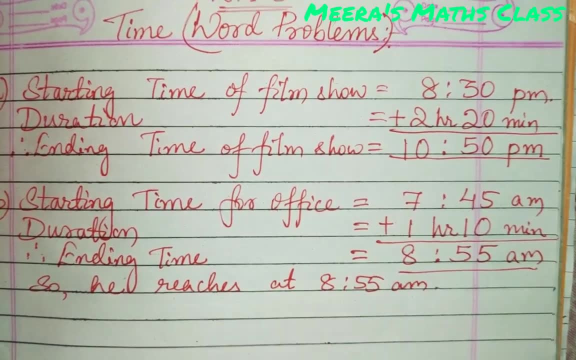 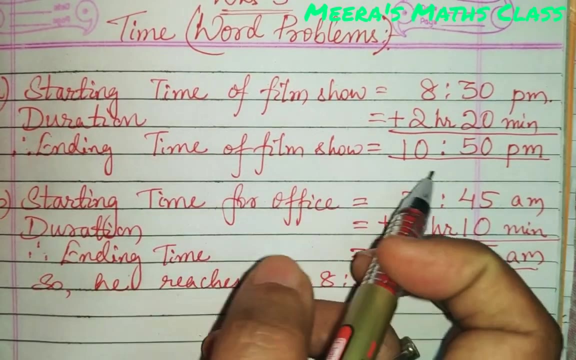 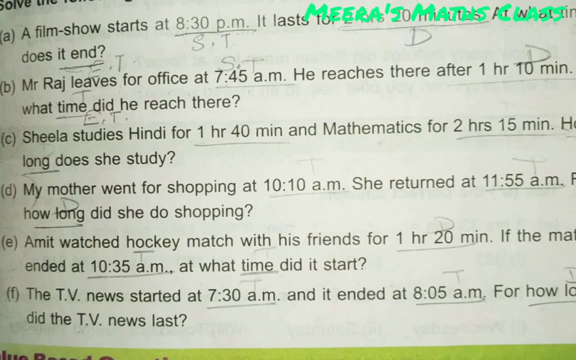 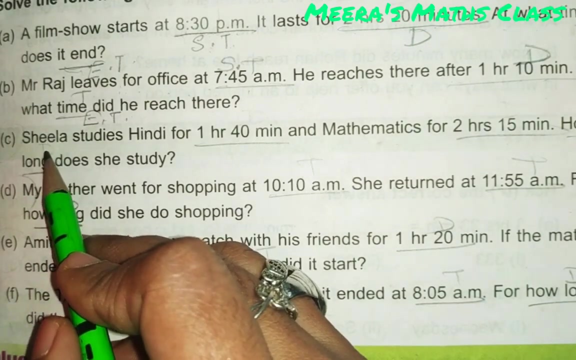 So he reaches that E to the To 855 in here also, you can write: so the film show ends at 1050 pm. you can write: or this much is also enough, okay, okay. now the next example, that is C number. Sheila studies Hindi for one. 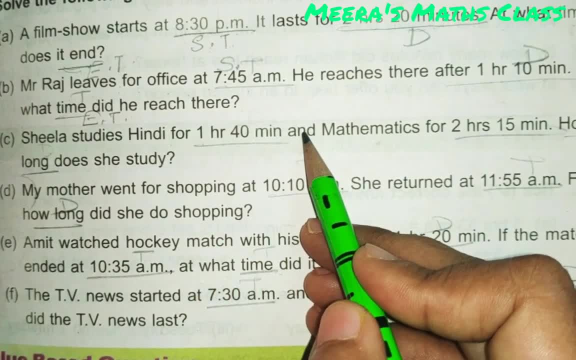 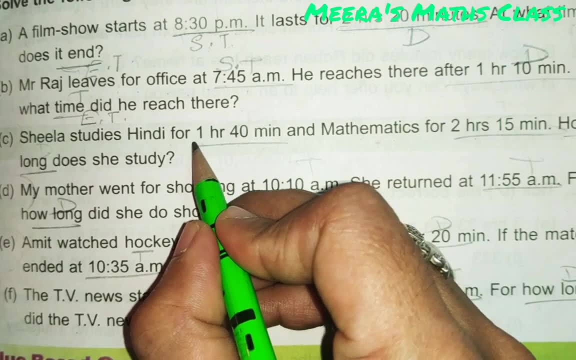 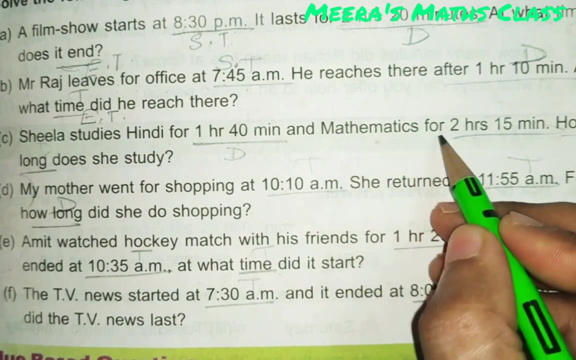 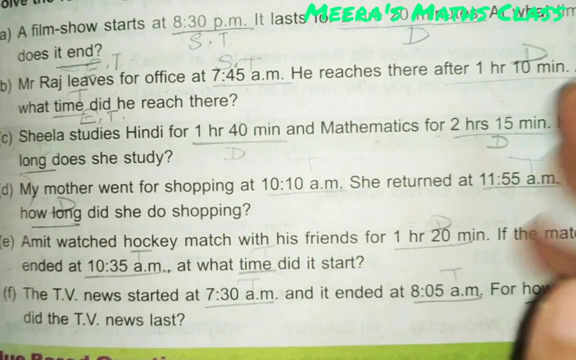 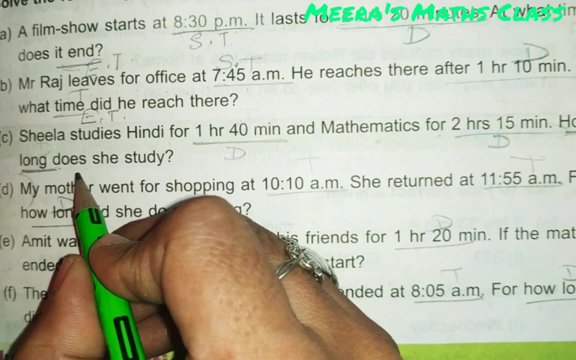 hour 40 minute and mathematics for two hours 15 minute. see, I underline one hour 40 minute. what is this? this is duration: mathematics for two hours 15 minutes. that is duration. so here two durations are given. durations of time is given how long. so how long does she study? so what? 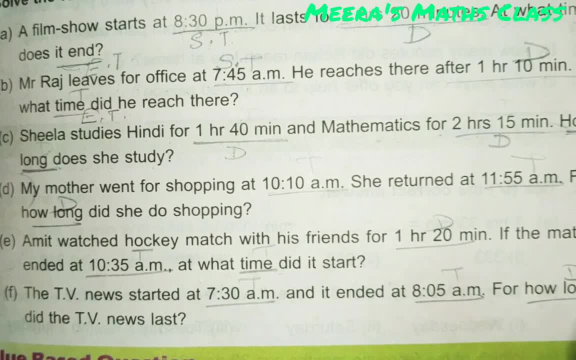 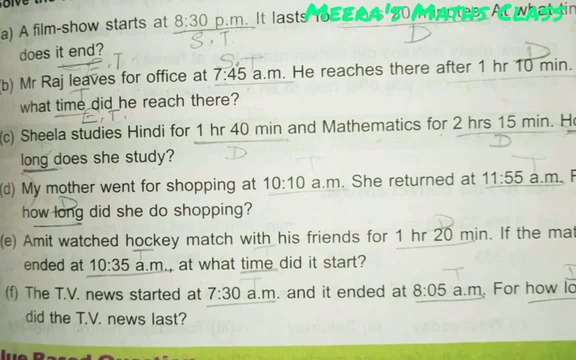 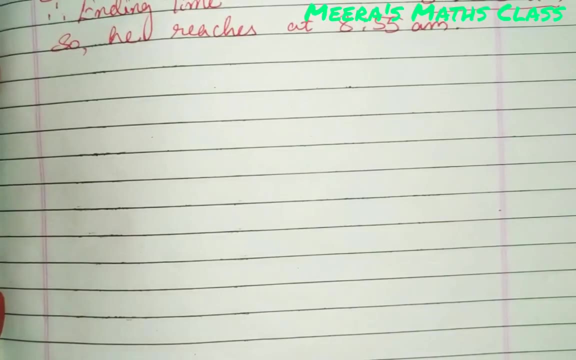 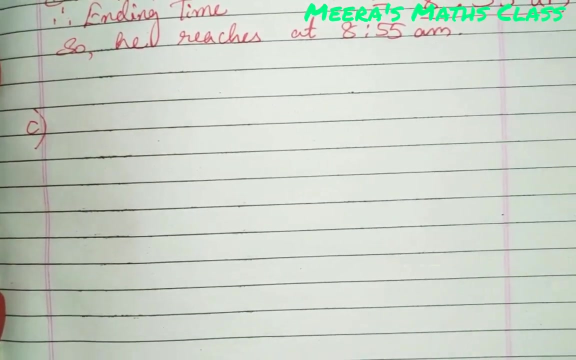 is asked how long. how long means it is asked for duration to duration times are given. now, if you add it, you will get the duration. okay, we will see how to write it. you leave two lines and then write the C number. okay, now what you are going to do. 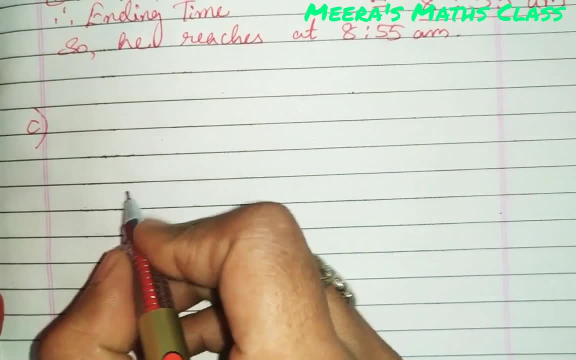 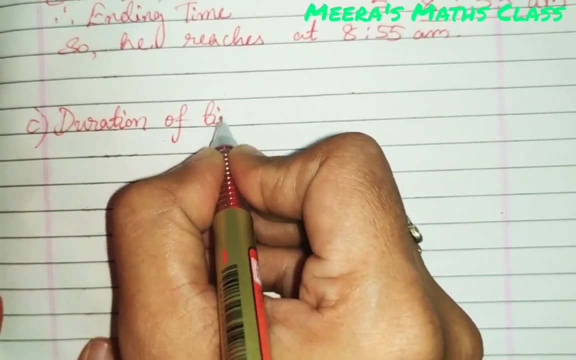 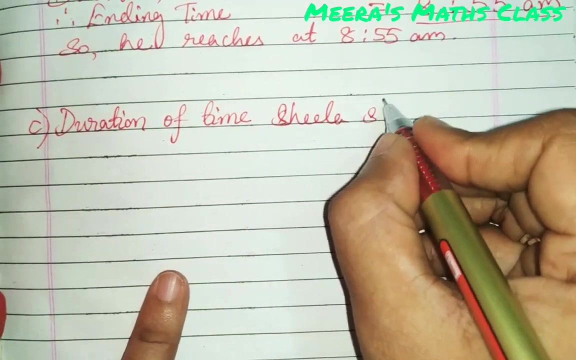 is right. first is duration of duration of time Sheila studies. you leave two lines and then write the C number. okay, now what you are going to do you write first is duration of duration of time Sheila studies. you leave two lines and then write the C number. okay, now what you are going to do you write first is duration of duration of time she. 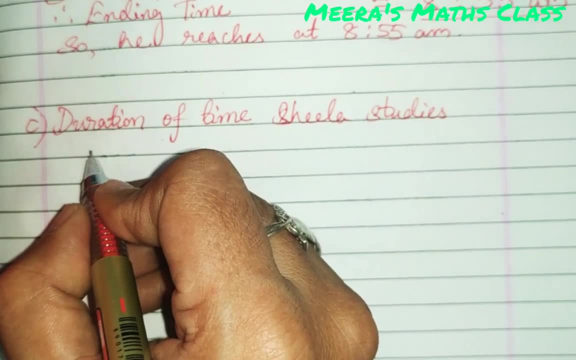 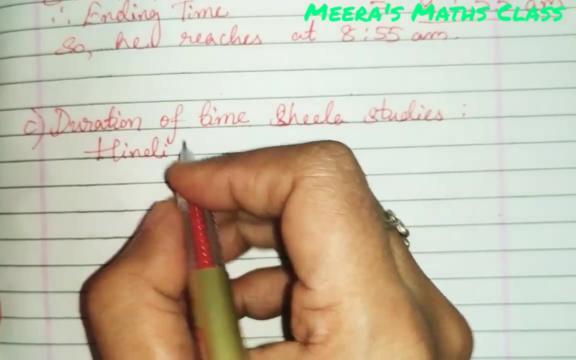 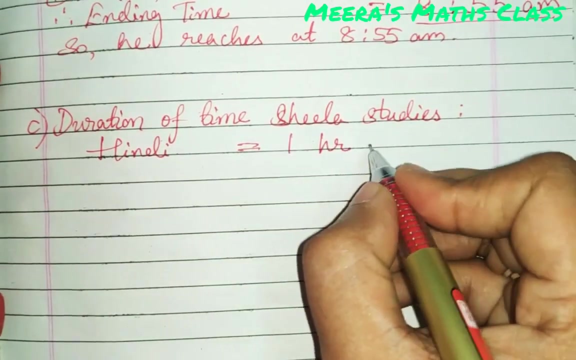 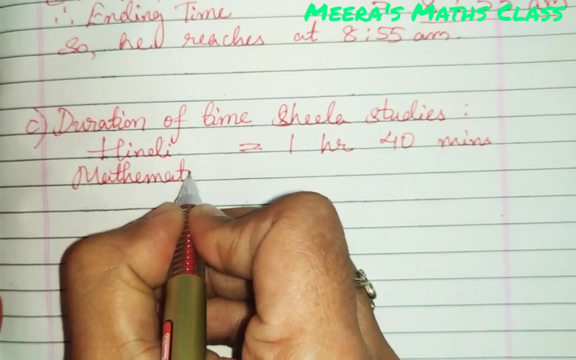 duration of time she. last. who is Hindi first is in the event last. who is Hindi first is in the event. who is Hindi first is in the event. that is in the amount one of a forty minutes. that mathematics duration. time time: Sheila. that is quantics. duration of time she. 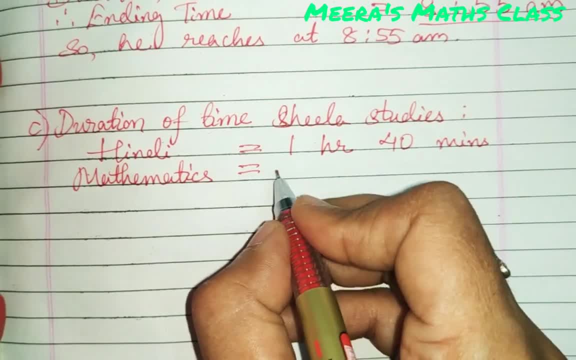 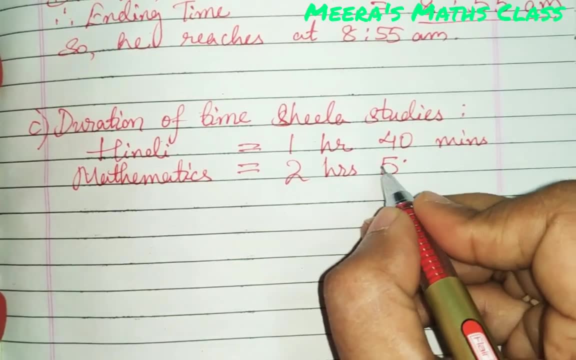 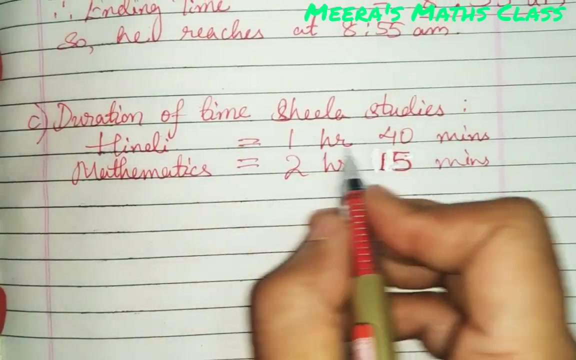 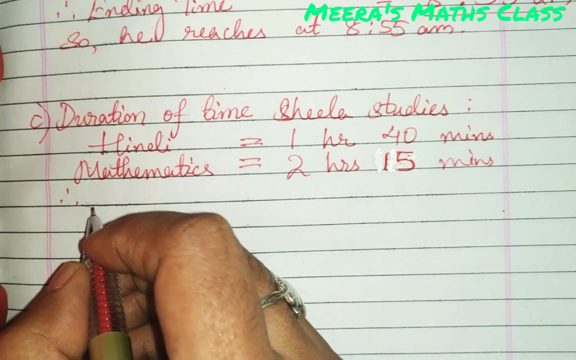 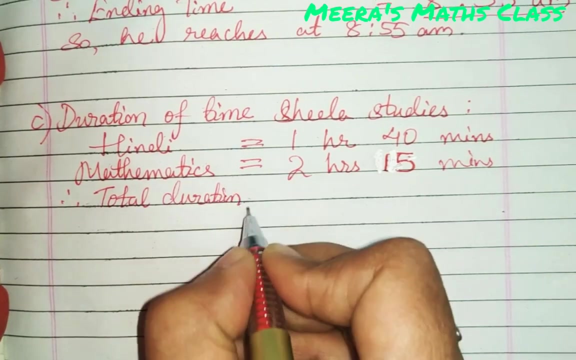 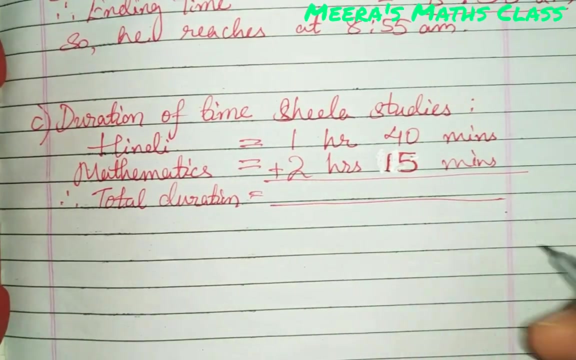 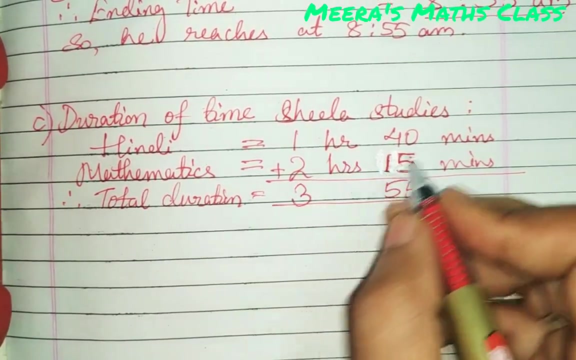 studies. mathematics is 2 hours 15. sorry, it's 15, this is 15 and so 15 minutes. now. therefore, total duration is equal to: we'll calculate the total time: 5, 4 plus 1, 5 1 plus 2, 3. now, here hours are given. your minutes are given. here it is 3. 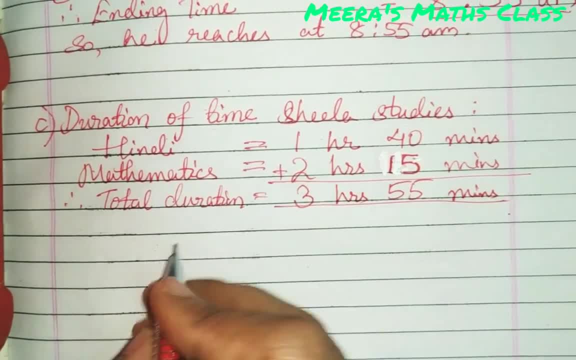 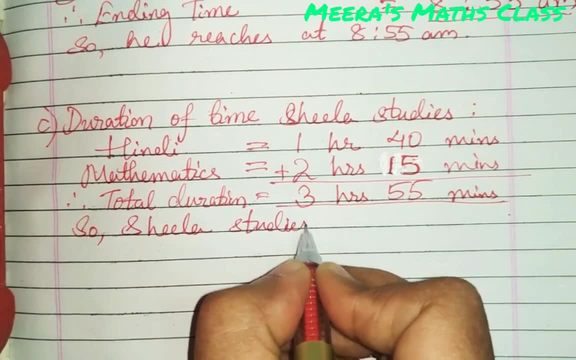 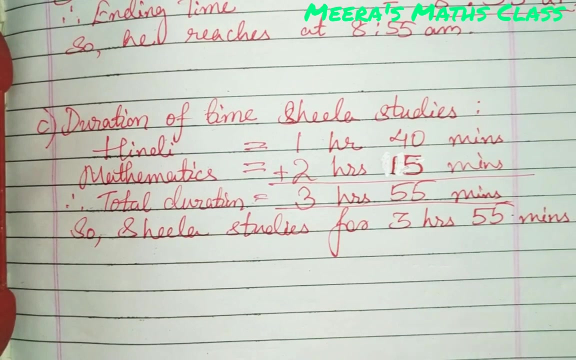 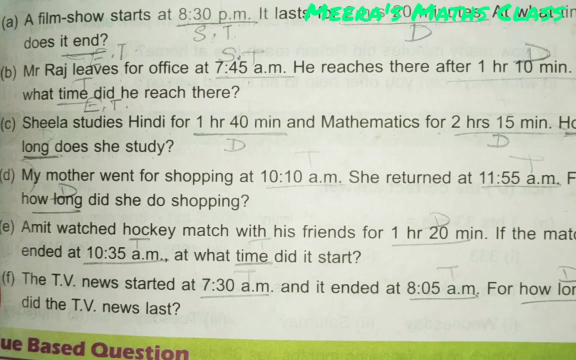 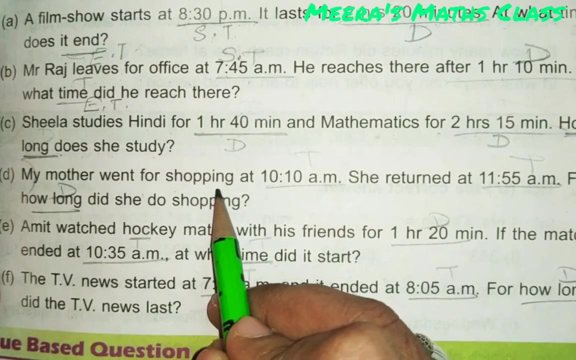 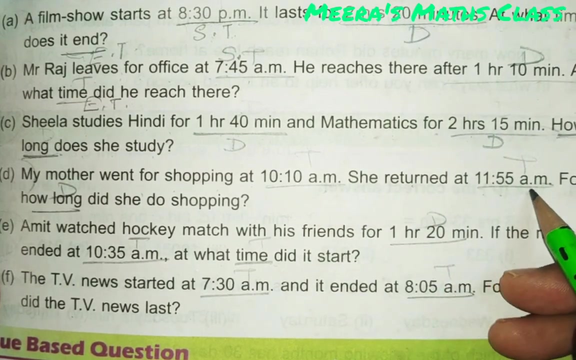 hours and 55, and then it's you can write. so: Sheila studies for three hours 55 minutes. okay, easy. now, children, let's go to the next question, that is D number. my mother went for sheila shopping at 10: 10 am. she returned at 11: 55 am. for how long did she do? 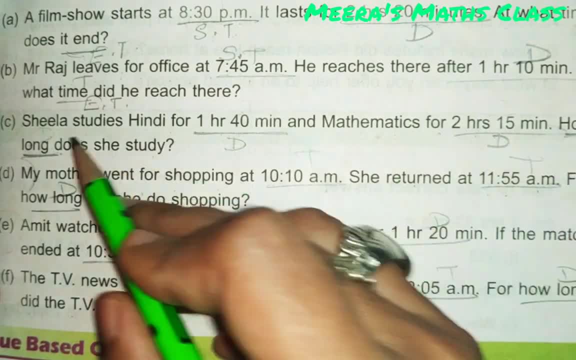 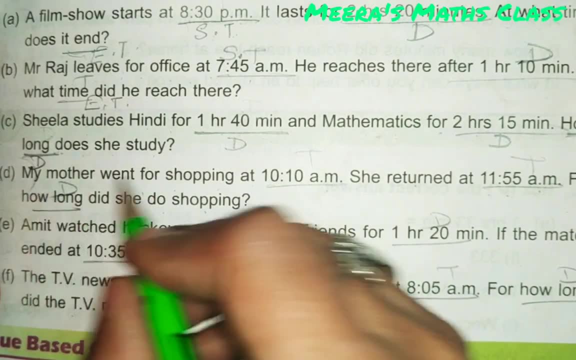 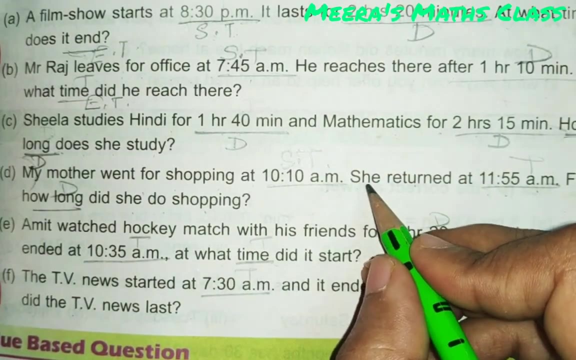 shopping here two durations were given. we found out the duration. this is how long that is duration we found out here. you see. another type of question is this: is the went for shopping at 10- 10 am. that means this is starting time, then she.